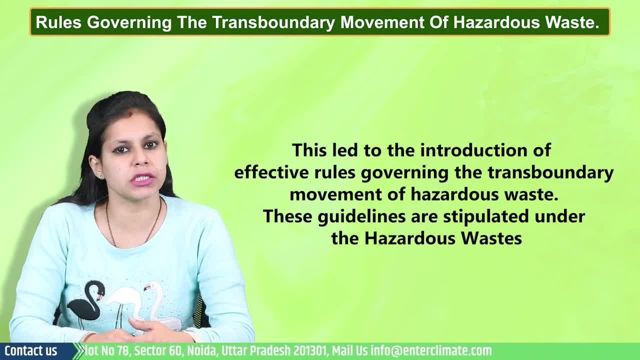 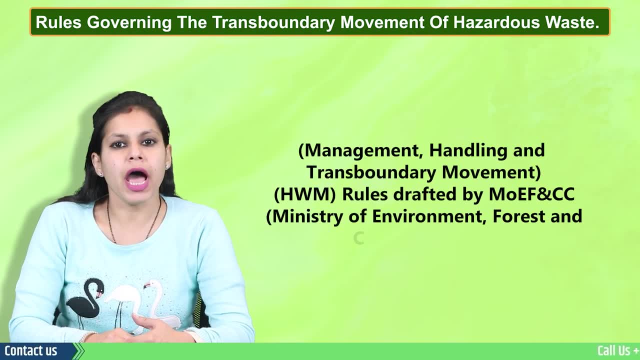 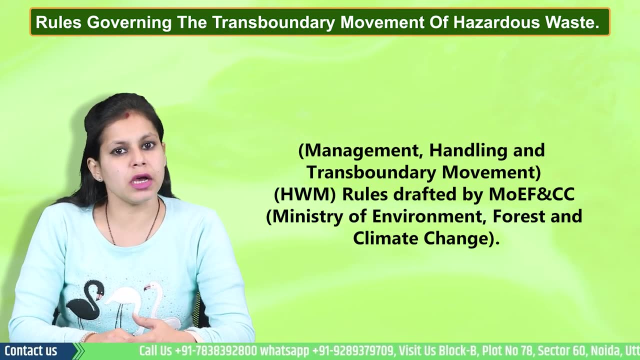 This led to the introduction of effective rules governing the transboundary movement of hazardous waste. These guidelines are stipulated under the Hazardous Waste Management, Handling and Transboundary HWM Rules drafted by MOEF and CC. So here here's a quick review of the rules governing the transboundary movement. 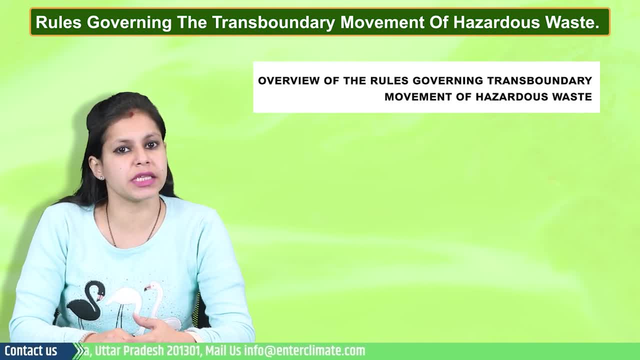 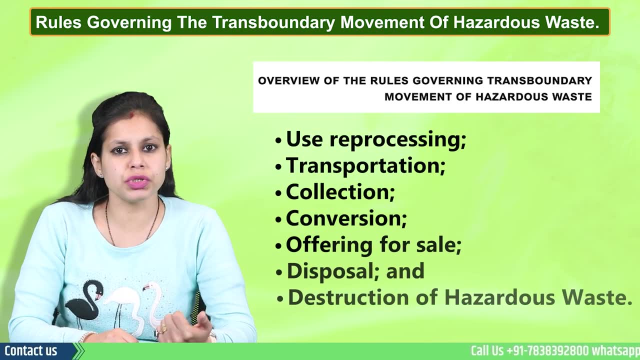 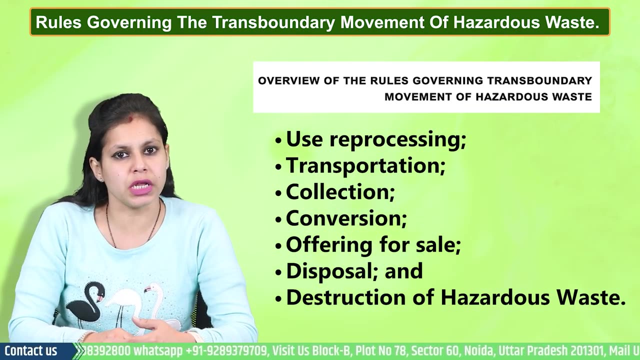 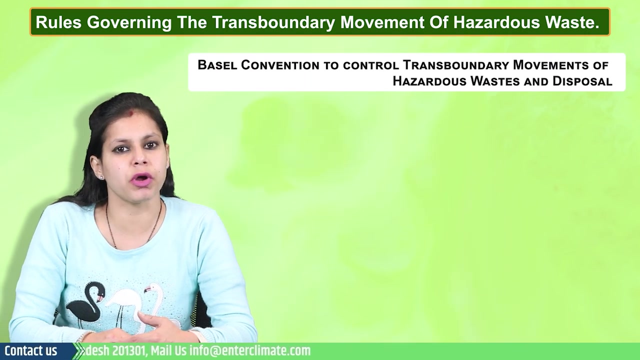 The HWM rules came into effect to guarantee safe generation, handling, treatment, processing, storage, package use, reprocessing, transportation, collection, conversion, offering for sale, disposal and destruction of hazardous waste. You might have heard of the Basel Convention to control the transboundary movement. 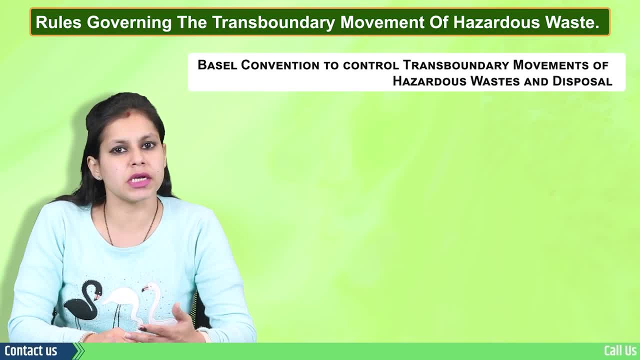 of hazardous waste and disposal. So now let us discuss in brief in this section of the video. The first inclusive attempt at regulating hazardous waste came in the form of the Basel Convention, which was adopted on 22 March 1989 in Switzerland. The Basel Convention aims: 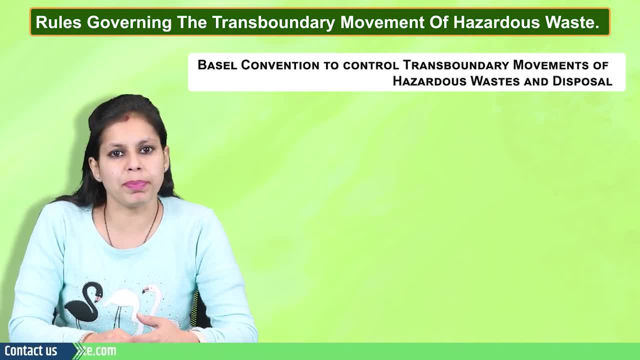 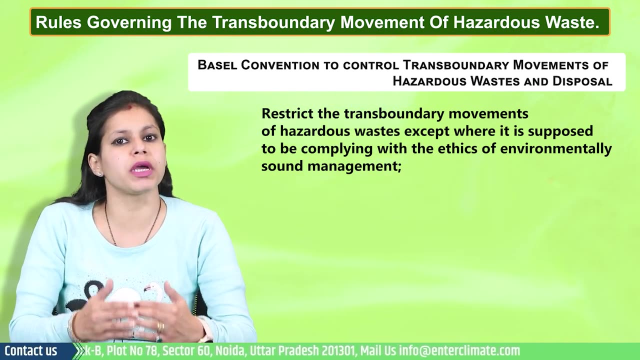 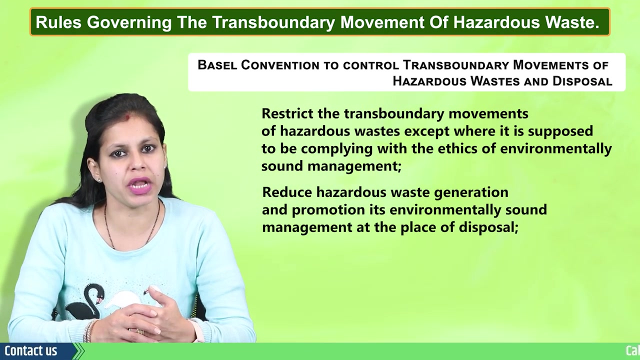 to protect the environment and human health. The scope of application of the Convention covers a wide range of wastes outlined as hazardous waste. The Basel Convention aims to restrict the transboundary movement of hazardous waste, except where it is supposed to be complying with the ethics of environmentally sound management, reduce hazardous waste generation and promotion. 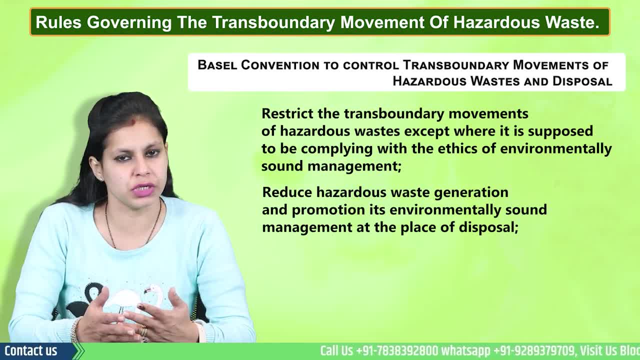 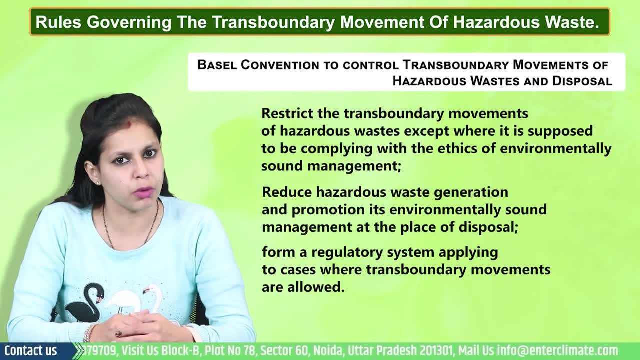 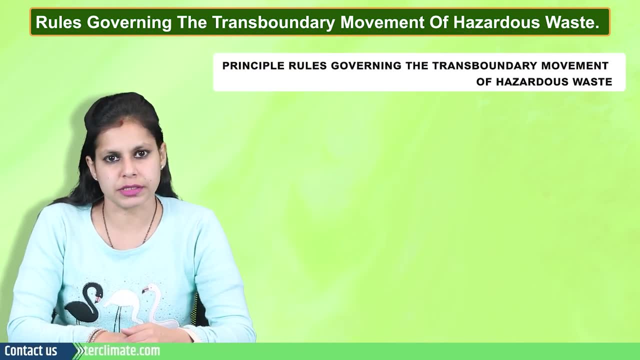 its environmentally sound management at the place of disposal and form a regulatory system applying to cases where transboundary movements are allowed. Well, so now I will be explaining the principal rules governing the transmission, handling, governing the transboundary movement of hazardous waste. 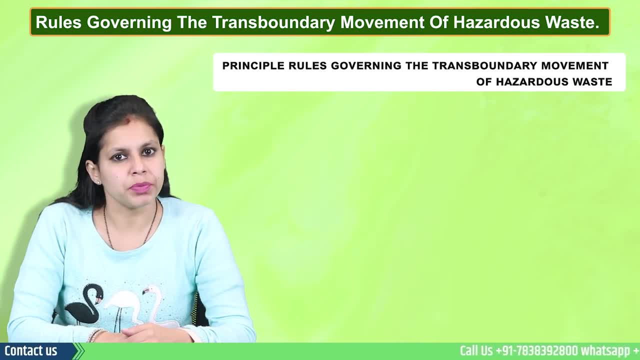 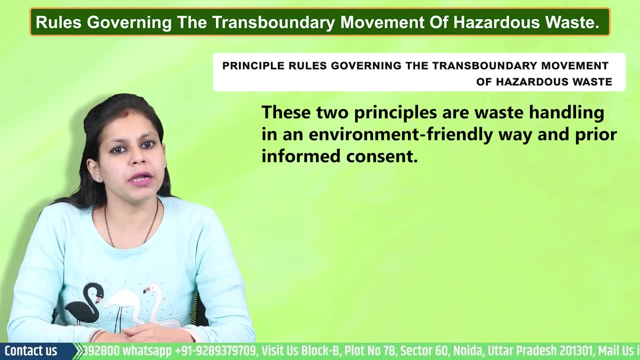 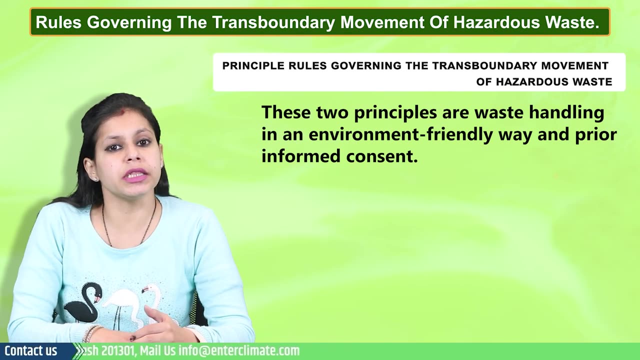 Lately, two main principle rules govern the things Defined in the Basel Convention. these two principles are waste handling in an environment-friendly way and prior informed consent. By stating an environmentally friendly manner, it is indicated that the waste must be handled proactively. 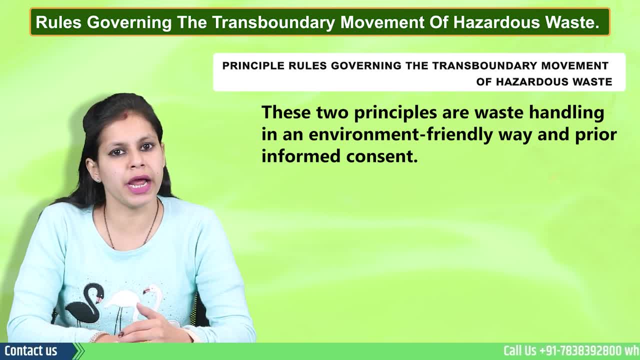 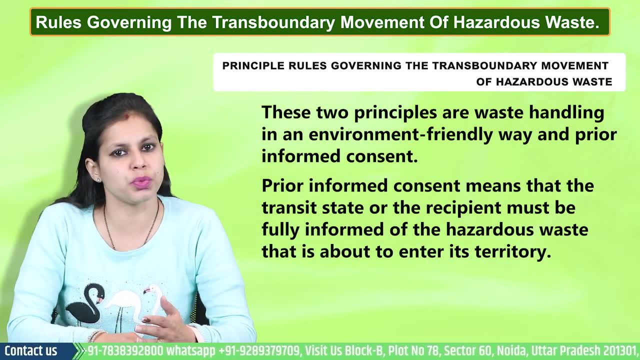 so that it doesn't harm the surroundings. On the other hand, prior informed consent means that the transit state or the recipient must be fully informed of the hazardous waste that is about to enter its territory. Also, it must accept such waste by giving its consent. 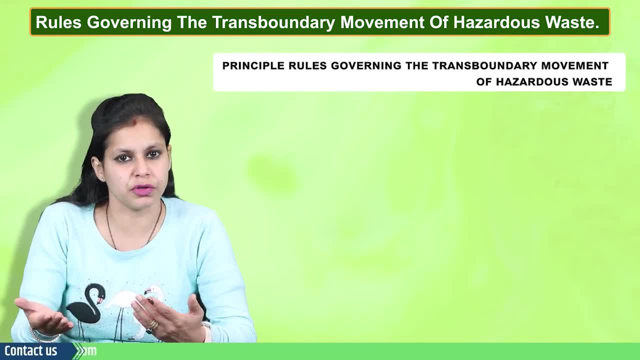 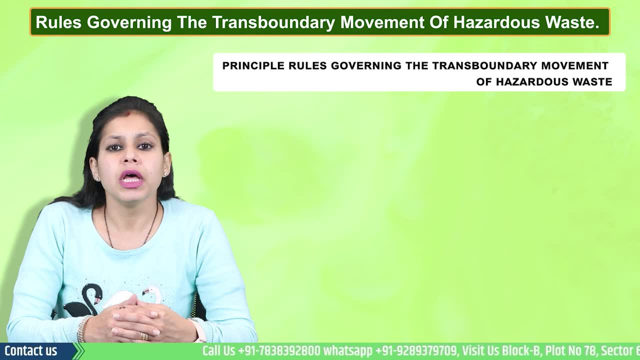 If this consent is not provided, the transboundary movement of hazardous waste isn't allowed. Also, the waste must be rebooted in case the decision is violated. Let us now discuss the cases where import and export of hazardous waste to or from India is illegal. 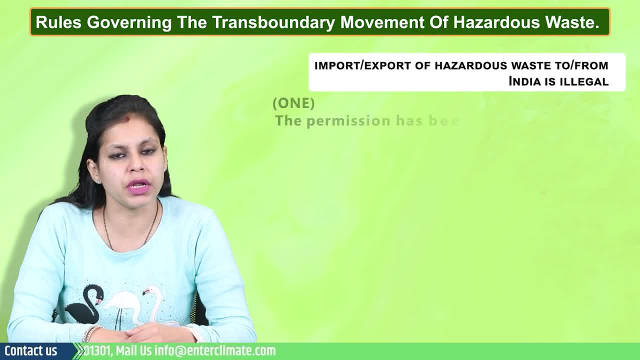 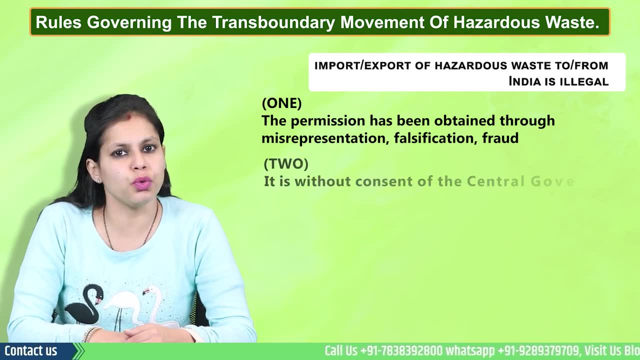 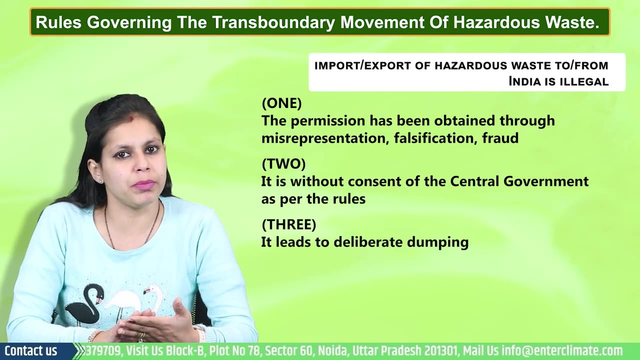 The import and export deemed is illegal if: 1. The permission has been obtained through misinterpretation, falsification, fraud, or 2. It is without the consent of the central government as per the rules, or 3. It leads to deliberate dumping. 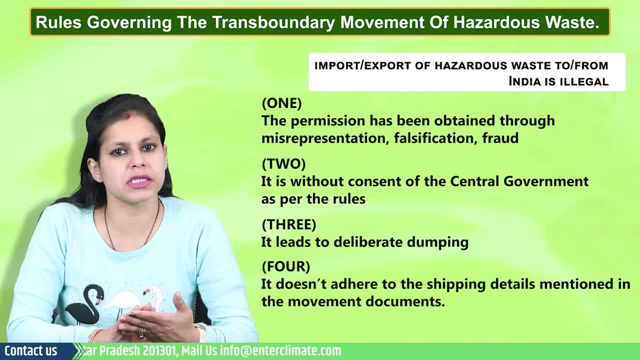 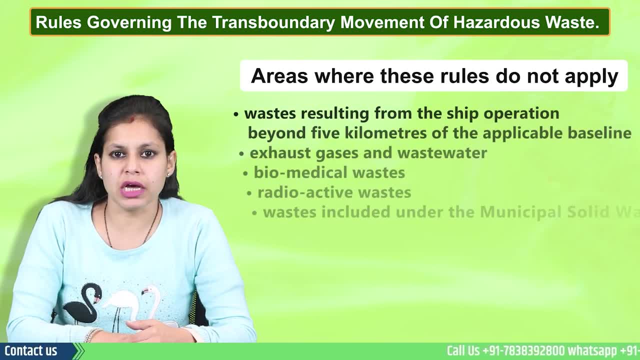 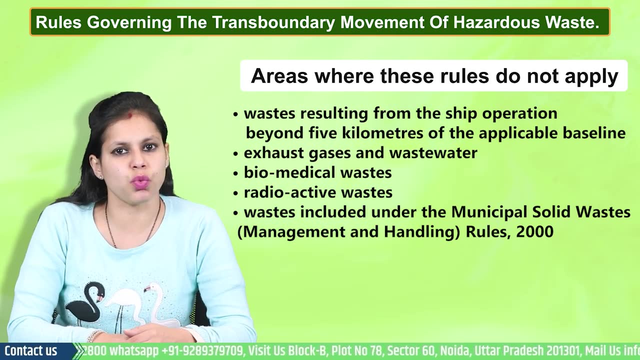 4. It doesn't adhere to shipping details mentioned in the movement documents. Okay, so now there are some areas where these rules do not apply. These are waste resulting from the ship operation beyond 5kms of the applicable baseline, exhaust gases and wastewater, biomedical waste, radioactive waste. 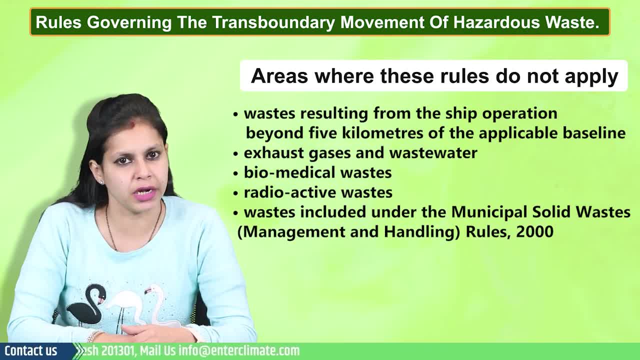 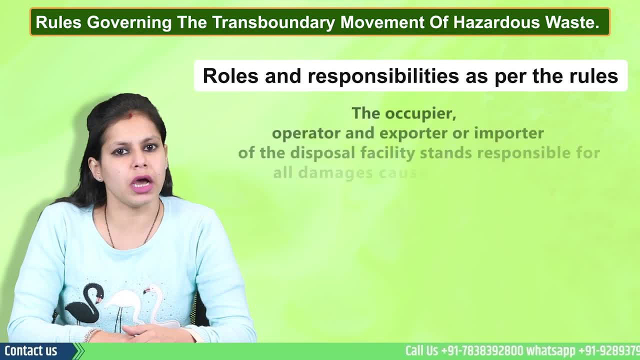 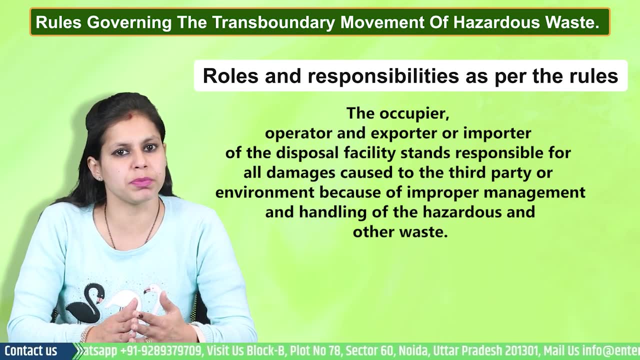 waste included under municipal solid waste management and handling rules 2000.. So here are the roles and responsibilities As per the rules, the hazardous waste of the copier operator and exporter or importer of the disposal facility stand responsible for all the waste. 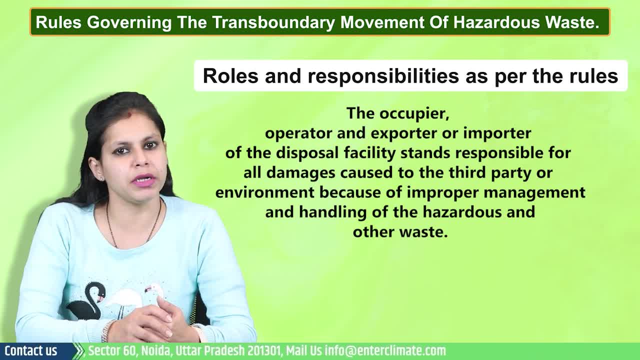 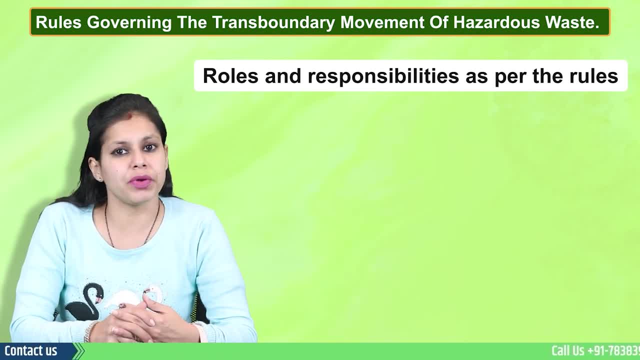 waste and waste that is stored in the generator or carry-on facility. Let us now discuss the goals and the solutions to these goals. all the damages caused to the third party or environment because of improper management and handling of hazardous and other waste. Every occupier engaged in generation handling. 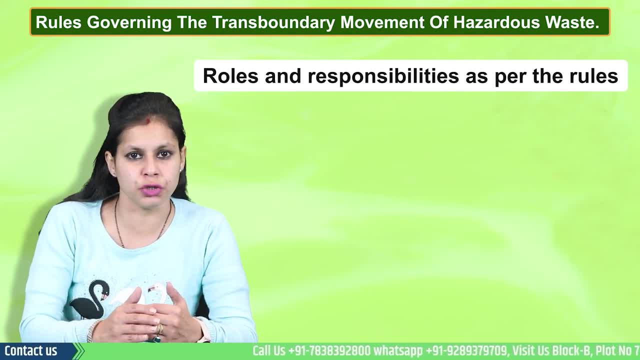 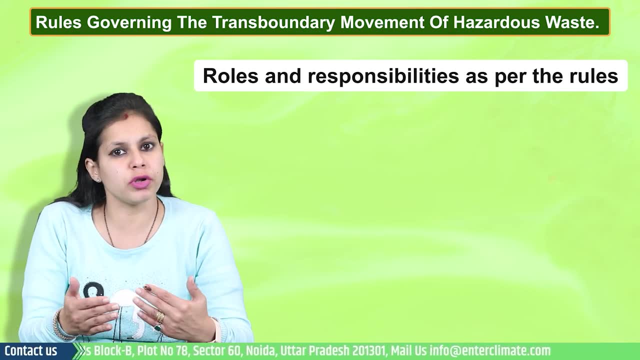 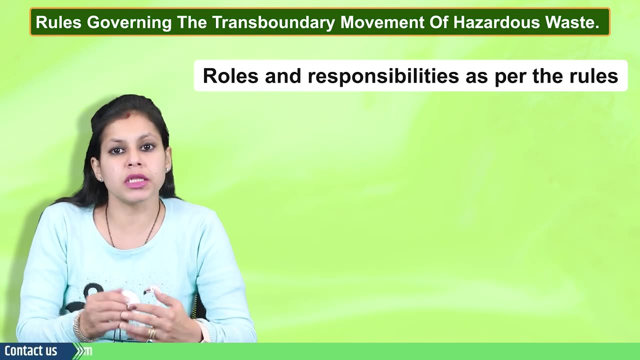 collection, packaging, storage, transportation, treatment, use, recycling, pre-processing, recovery, processing, utilization, offering for sale, co-processing, disposal or transfer of hazardous and other waste must apply in Form 1 to the SPCB. This must be done to obtain. 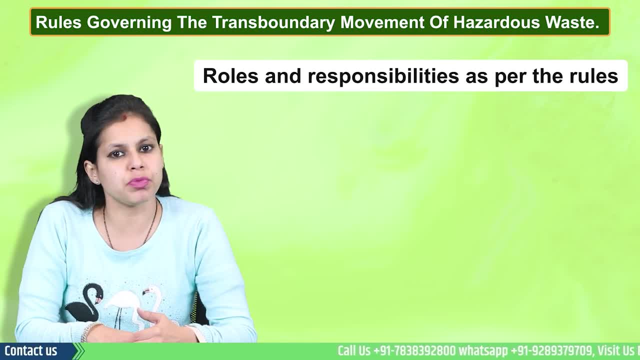 the authorization mandated by the rules governing the transboundary movement of hazardous waste. The authorization must be obtained within 60 days from the date of rules publication. Also, MOEFNCC is the nodal ministry to deal with the import and export of waste. accordingly, 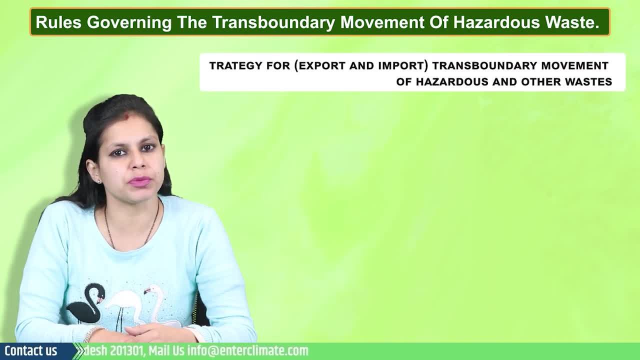 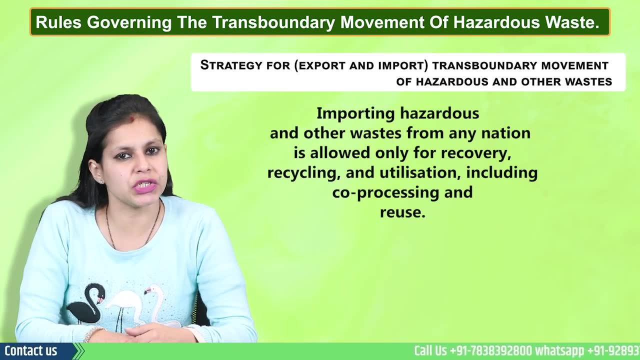 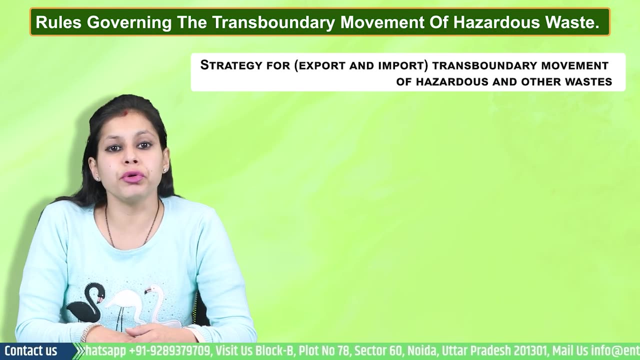 Well, now let us talk about the strategy for import and export of transboundary movement of hazardous and other waste. Importing hazardous and other waste from any nation is allowed only for recovery, recycling and utilization, including co-processing and reuse. No transboundary movement of hazardous.